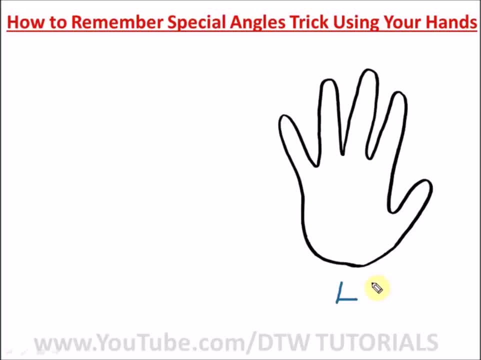 through. look at your left hand, face it towards your face. okay, and tag this particular as your, your thumb: the small, the smallest, as what zero degree, this would be what 30 degrees, this would be 45 degrees and this would be what 60 degrees, and this would be the little finger down here. 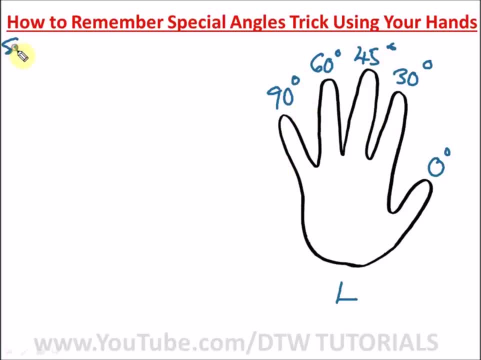 would be what? 90 degrees. okay, so let's say we want to get our trigonometry, that's our trigonometry ratios. uh, for course, and also for tan. let's say, for example, we want to do 60, that's going to find sign 60. 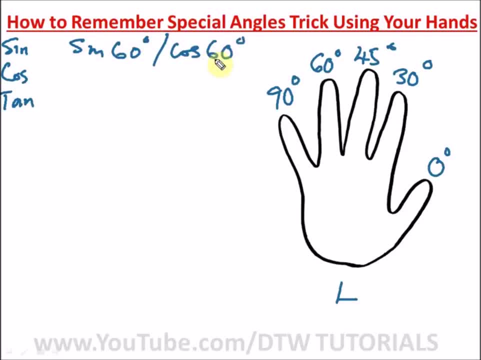 degrees and cause 60 degree. we're going to do it together. okay, so this is the finger for 60 degree, right, so you cross it out. then on your left side. your left side will represent your sign side. okay, why the on this? the the right side of the 60 degree will present your word course. 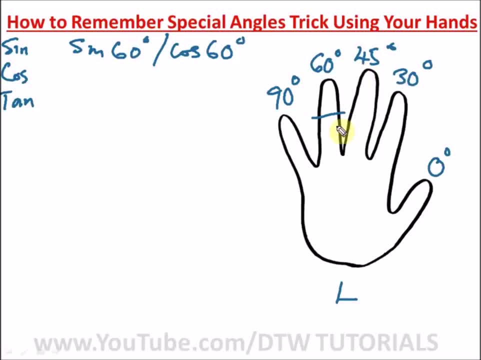 so for to get your sign 60, we'll count remaining fingers on our left side. so we have one, two, three, so that's three, so we write down three, then we square root- it's always square root and we always divide by two. so you can see how easy this is. so the sign of the trig ratio of sign 60 is: 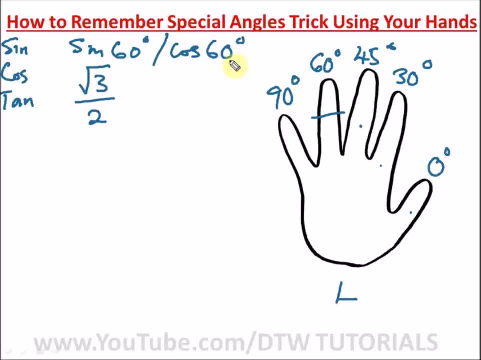 what square root of 3 over 2.. now let's do four costets for cost 60.. how many fingers left here? we just have one, so we have four fingers. we're going to divide by two and we're going to divide by two. so we have what one will square root it and divide by two, and what is the square root of one? 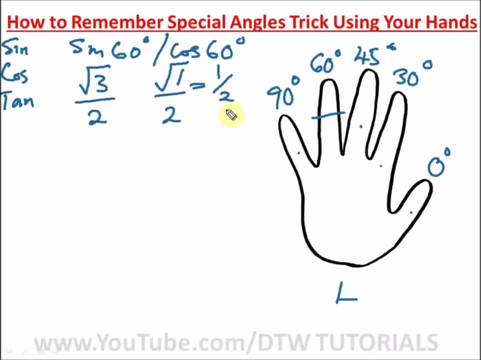 is still one, so we have one over two. so the trigonometric, trigonometric ratio of cost 60 degree is what's one over two? that is what half. okay, let's do another example. let's say we have sign 30 degrees and cost 30 degrees. okay, you know, you could do this um on your rough sheet. 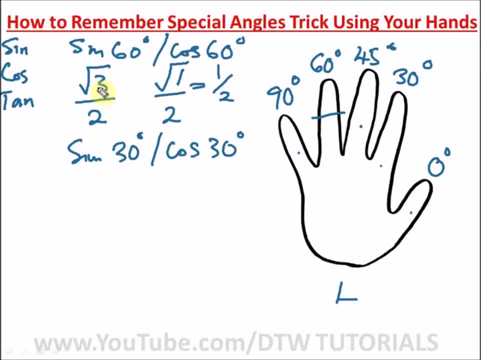 immediately you enter your the exam hall. just quickly do this, right, write all this down so you'll be easy for you, uh, to calculate. okay, just put it as one of your- oh, your- trigonometric ratio. immediately use your hands, get it down so it'll be easy for you anytime you want to solve you just 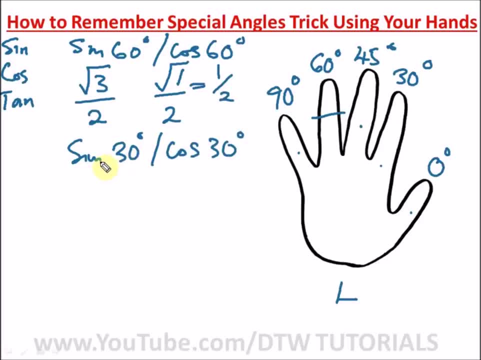 look up and you use it, okay. so for your sign, sign 30 degrees, we'll cross the 30 degrees. uh, fingers out, okay. and what is left on our left side to look for our sign? we go towards the left side. we have just one finger left, so we have one, the root of one. we have one finger left, so we have one, the root of one. 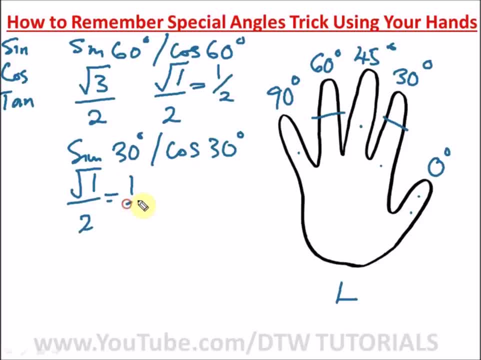 square root of 1 over 2. and what's the square root of 1? it's still 1 over 2. so to get your cos 30 degrees, what do we do on our right side? we count 1, 2, 3, so we have three fingers left, so we: 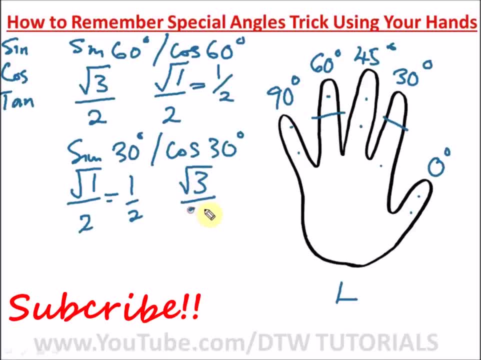 have what 3 and the square root of 3 divided by 2, so you can see how easy this is. now to get your tan. remember that what tan is what sine over what cos? okay, so let's say we want to find tan 30 degrees. okay, so to get tan 30. what's your trigonometry ratio of this? so you are going to. 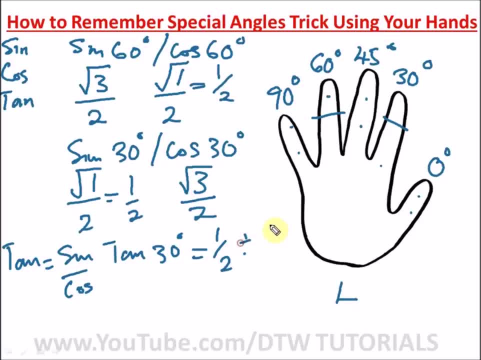 just divide 1 over 2, divided by what root 3 over 2. okay, and what would this give us? this is 1 over 2 times 2 over what root 3, and when we cancel, and what is tan 30 degrees? tan 30 degrees is what. 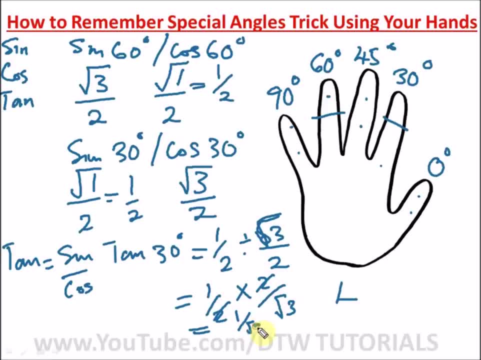 1 over root 3. you can see how easy this is, so that is how you can just remember your special angles using your hands. all right, so thank you for staying tuned to today's, friday's, mastery. please try to share this uh to your friends also preparing for exams. this is really going to help them, and also when you 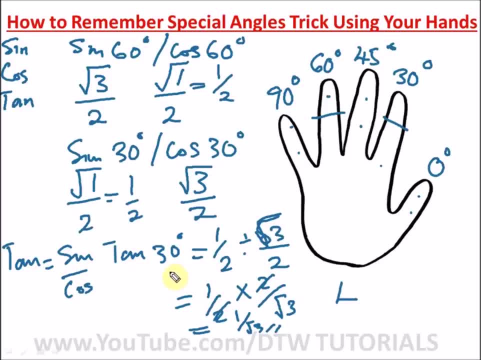 enter the exam. if you're a math student writing a math in your jam, just immediately write these special angles, do this trick with your hands, put it down one place so it'll be easy for you to solve all right. so thank you for staying tuned to today's friday's mastery, and you are destined. 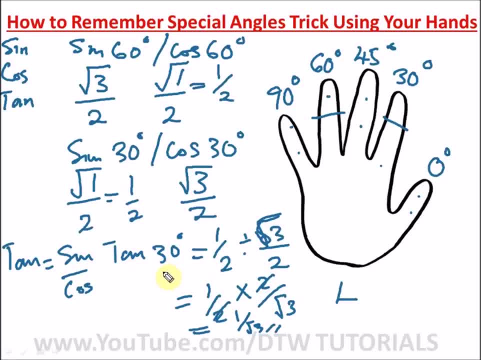 to win. don't forget to subscribe, like and share, and remember jesus christ is coming soon. give your life to christ. you are destined to win. bye and success in your exams.